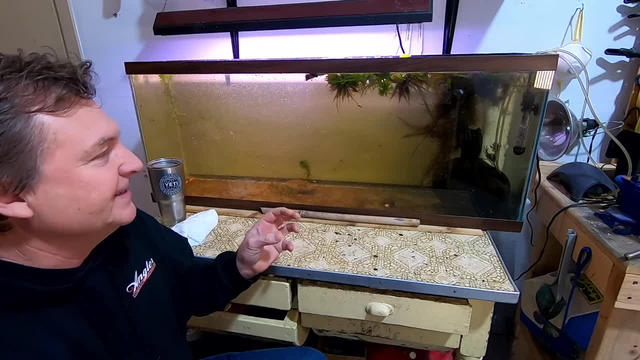 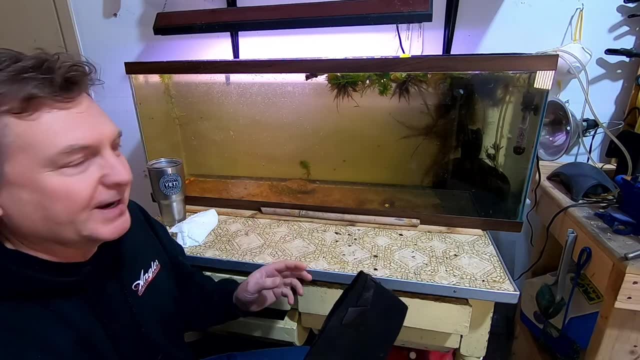 not going to work for you. You could put sponges over the intake, but still the Daphnia get pushed into that, And I did try that at the beginning and it just didn't work out. So what I came up with? 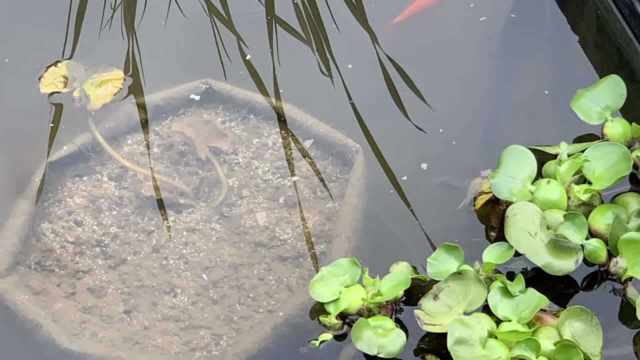 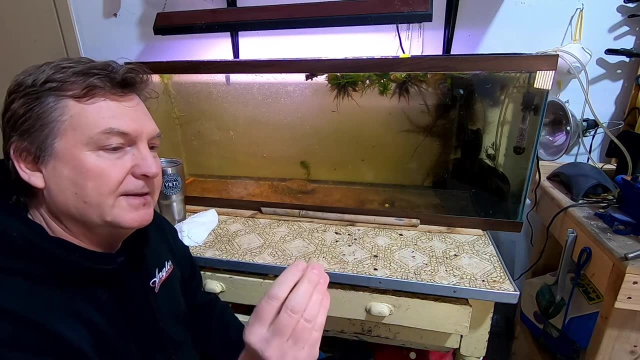 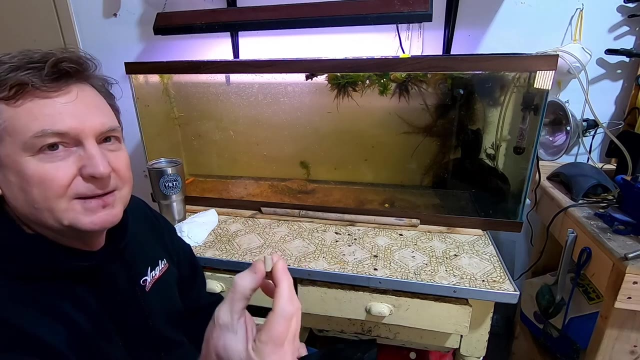 like a flower pot for aquatic plants, a three gallon flower pot bag, I guess. I'm not sure exactly what you're supposed to call them. So what I did was take a whole bunch of these little filter media ceramics and it just kind of looks like a bone, but you know how bones have a lot. 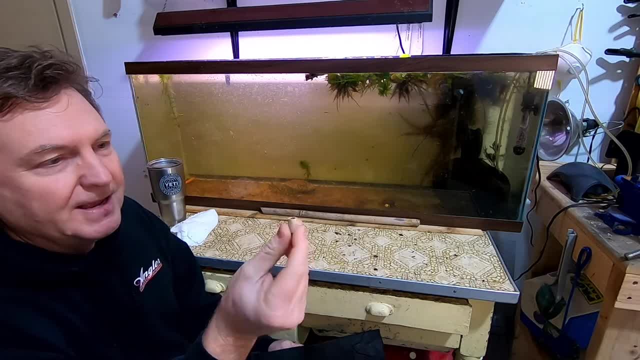 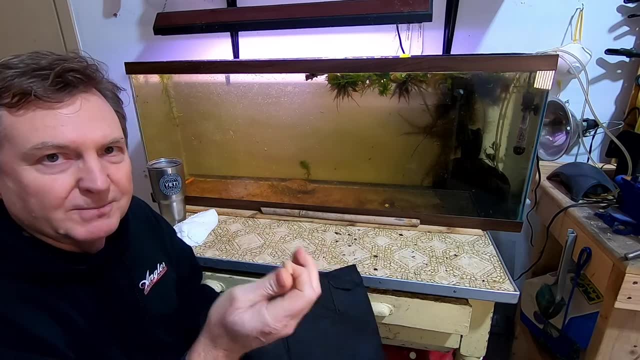 of pores in them. Well, this is a similar type of structure. Within this are millions and millions of little pores and just a ton of surface area places for bacteria to grow. In fact, I pulled this one out of the tank. There's another one there, since it's got loose. 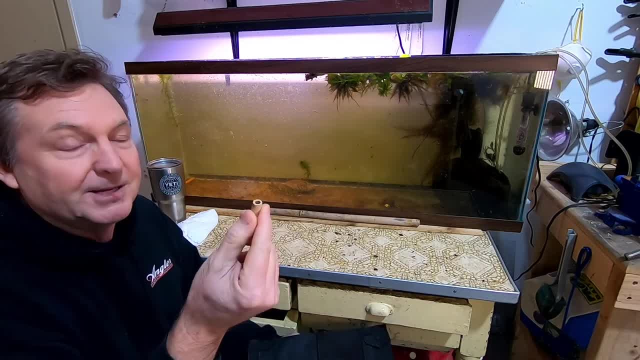 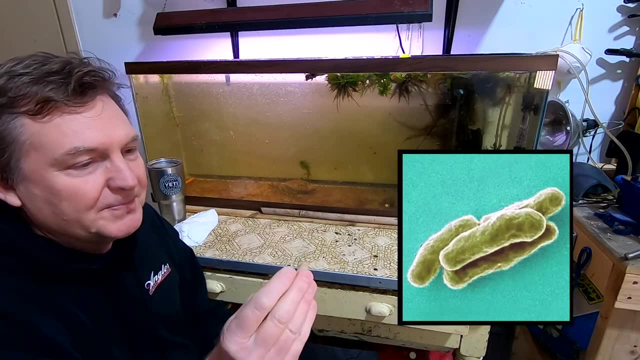 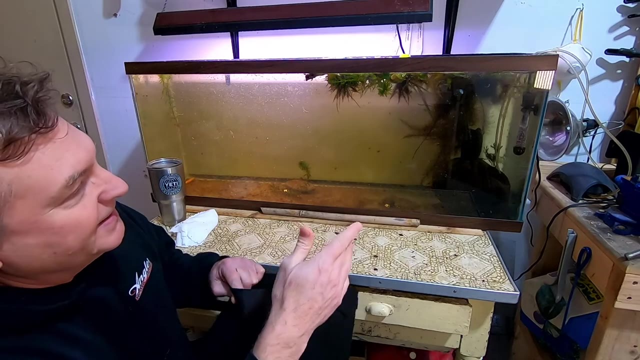 when I was making it. But on this there's you know who knows how many, but millions and millions and millions of tiny little bacteria. that does the nitrogen cycle for you. So that's what I filled it. put it in the bag, put this guy back in the water. Now the air pump. the point of that. 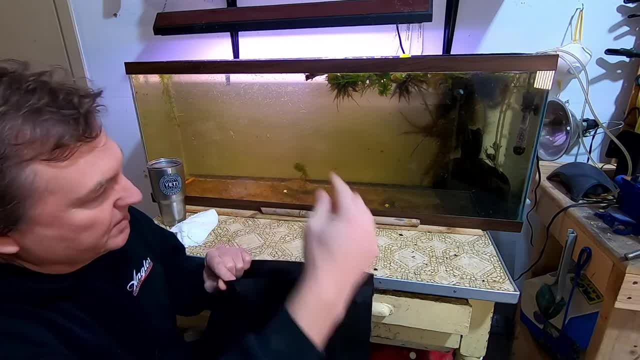 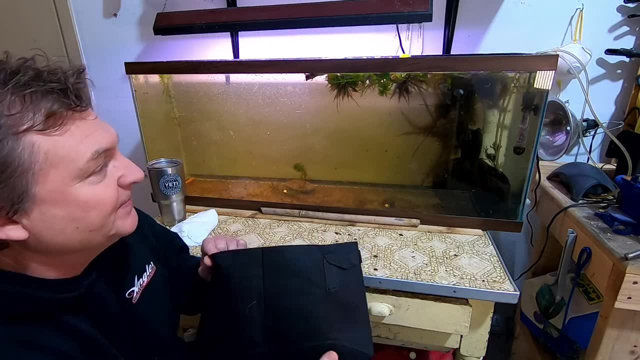 besides aerating the water, is to get the water to flow through the bag and through all that media to feed the bacteria. Basically, you can think about it that way. Now you can see that those bubbles are pretty big and it's working. It's been working like this for. 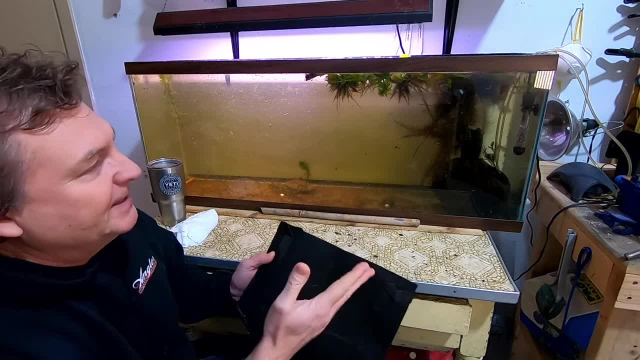 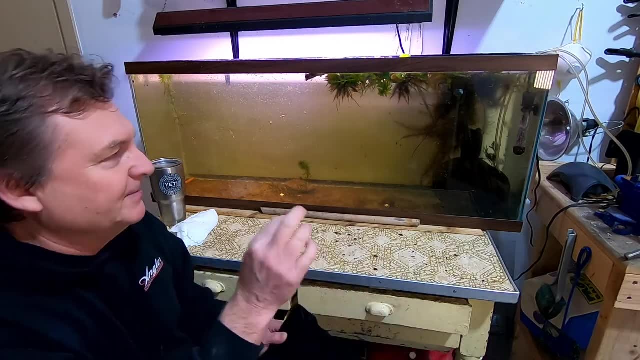 a long time. And you know, if it's not broke, don't fix it. But next time, whenever I do tear this apart and then maybe clean the filter or kind of get it going again, I'll put some airstones on the airlines there and get some finer bubbles. I think that'd be a better way to go, but it's. 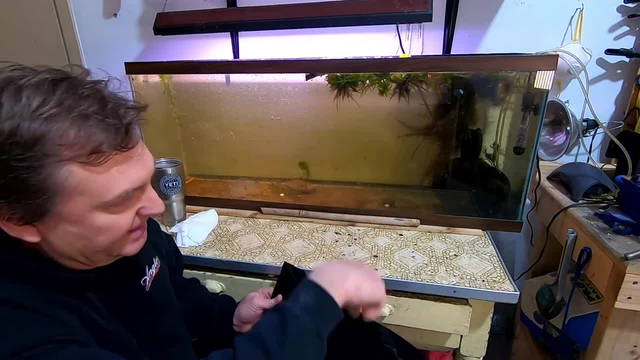 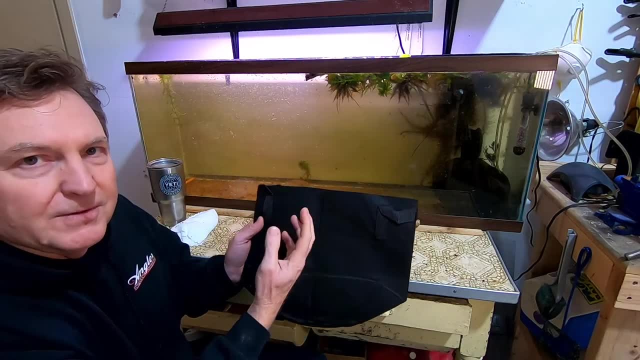 working fine, just like this too, But all it is is two airlines. a lot of them are very small and they're very, very big in size, And so the problem with this is that you can't get that air down into the bottom of the bag, So it's forcing air to to push that. 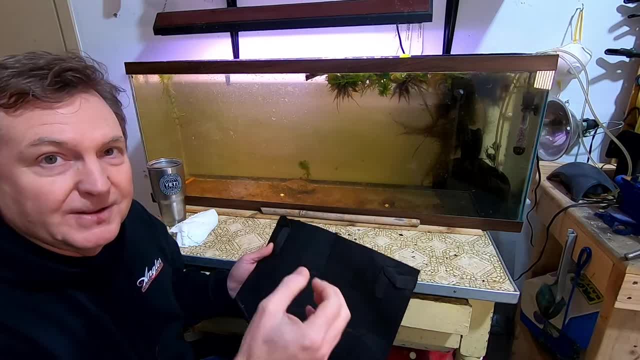 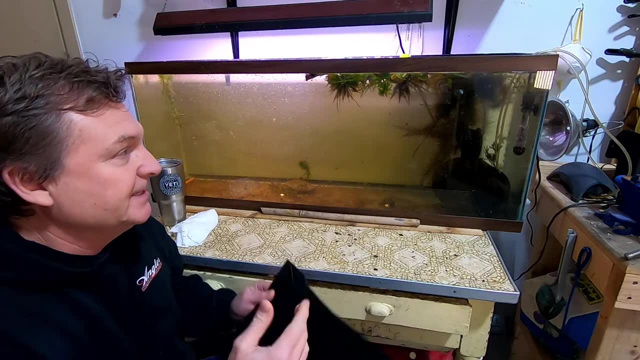 water up through all the filter media And that works really well And I get that idea from what would probably be. the ideal way to go would be a sponge filter, where you've got air like that just pushing the water through the sponge and all the bacteria lives in the sponge And that's a 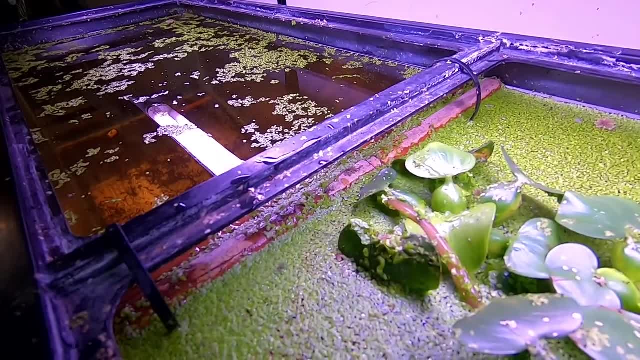 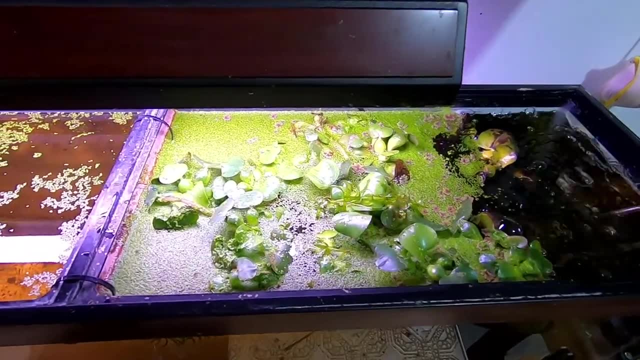 really great system that's used a lot for shrimp. i'm real happy with it. the plants i've got- duckweed in there, which is a great filtering plant, grows like crazy, and also some water hyacinth, which is a great filtration type plant and also a reason. why i've got the water hyacinth in here is i'm trying to keep it alive over the winter because hyacinth is from the amazon originally, i believe, and and the stuff you know, if you leave it out during the winter here in the northwest it's going to die off. it might make it through the. winter, but it starts looking pretty ugly so i keep it in here. it's under the light, it's doing well. in the spring i can just put some back out in the pond and have some water hyacinth out in the pond, but they are amazing little things. they're also called water fleas. maybe you had them when you're. 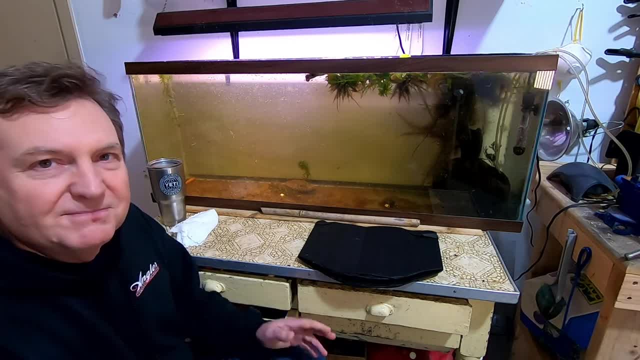 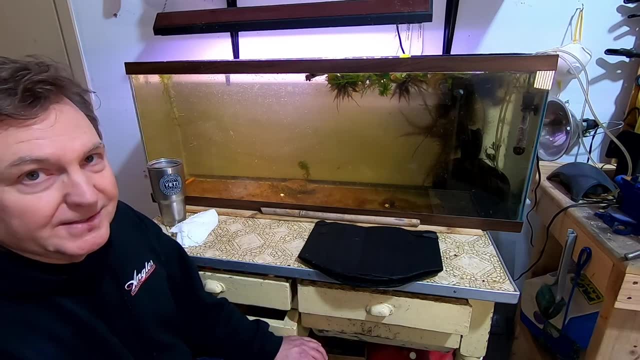 a kid- maybe you did a in schools- you know it's to do little projects with water fleas. those are the daphnia. if you fish lakes, like i know shasta lake, northern california is completely full of daphnia and lots of lakes are. and these are the magnolias. 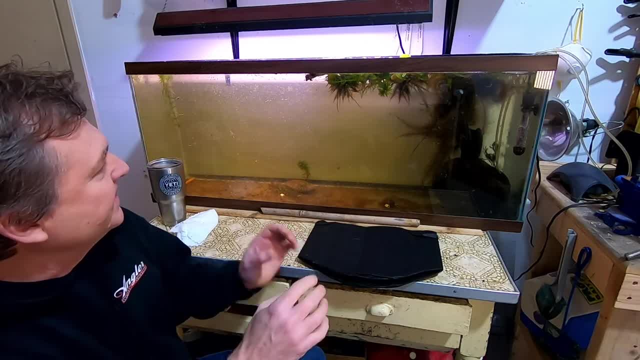 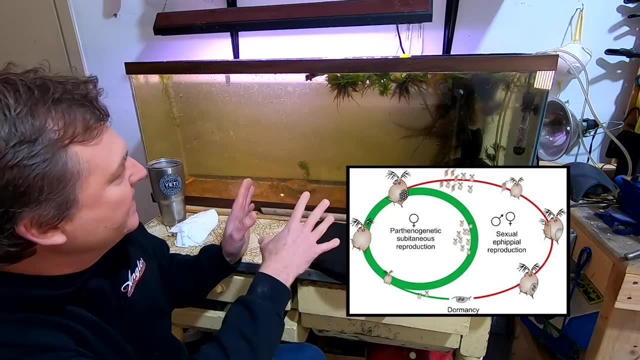 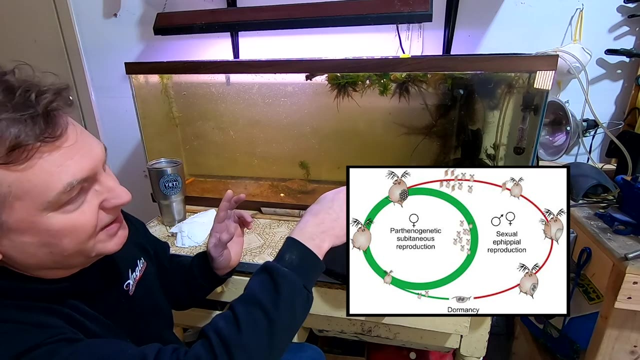 though the big ones, and the way they reproduce. it's kind of interesting. they they reproduce both sexually and asexually. so right now, these guys being kept like this, they're not going into their, their dormant stage, so to speak. i do have a little heater in there. 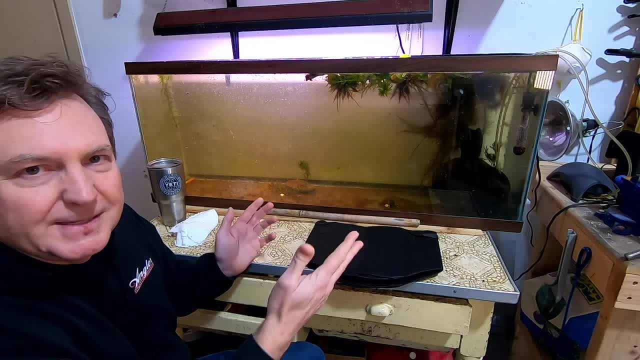 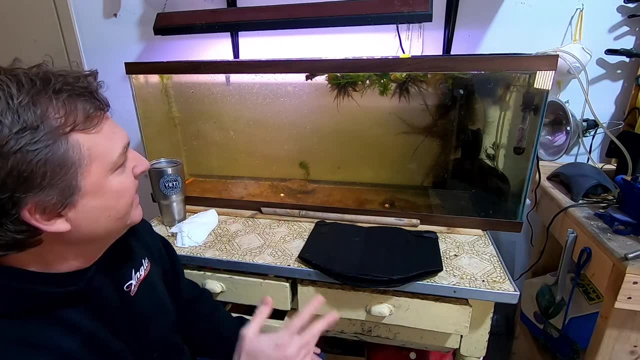 i keep the water right around 68 degrees. that seems to be good, but i've had them down a lot colder. i've had them a lot warmer. they seem pretty happy with it all and- and even with the colder water- it was getting down close to 40 degrees- they were still reproducing as long as they have food, it seems like they'll reproduce. they're pretty much all females right now in this particular species and in this stage each one of these guys can produce inside of them like a hundred eggs, and then those eggs hatch inside of them. so you can imagine how small these 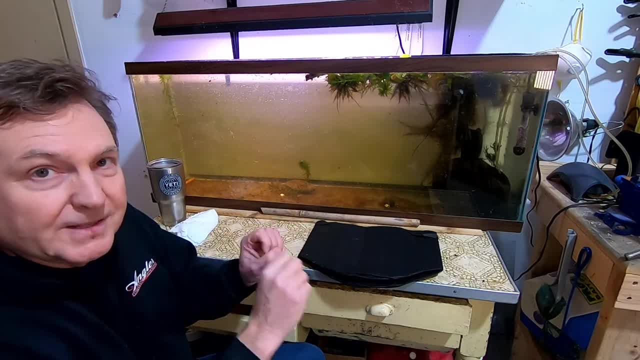 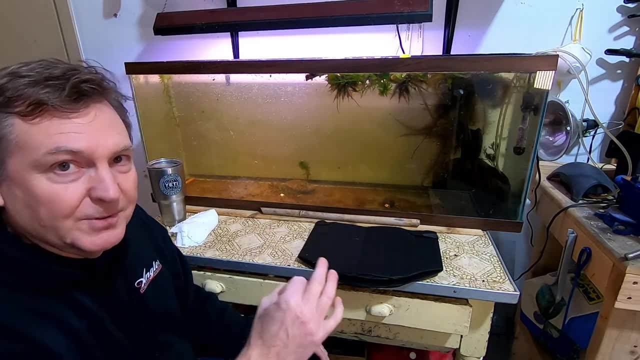 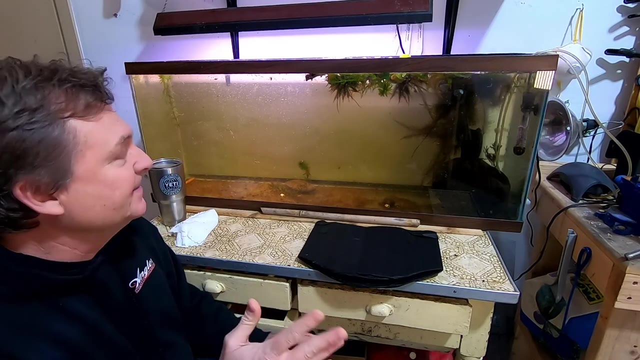 guys are, and then they release those rather quickly and it's only a less than a week process. so it's a amazing. so you can have: one daphnia can produce a hundred daphnia, and those hundred daphnia are each going to produce a hundred daphnia within less than a week. so this is a you know you talk. 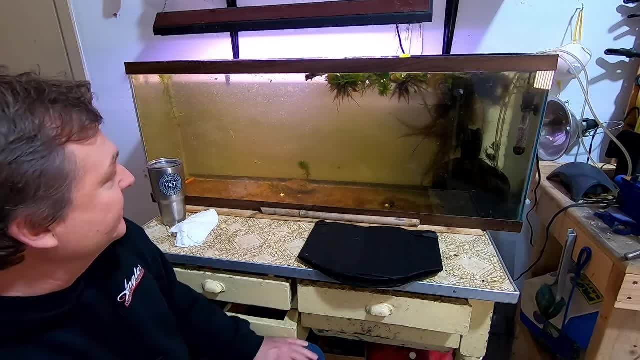 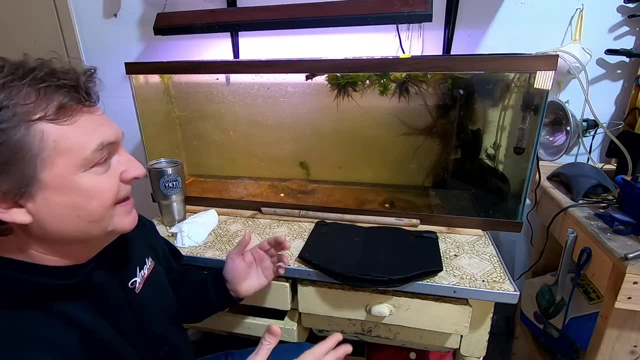 about rabbits. what these guys got got it going on for sure when it comes to reproduction. so food is incredibly important to these guys. no food, no daftion, you know, and, like i said, they're down. from what my experience here, they don't seem to be so sensitive to. 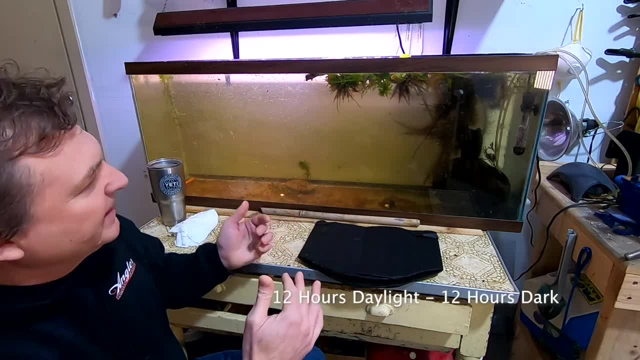 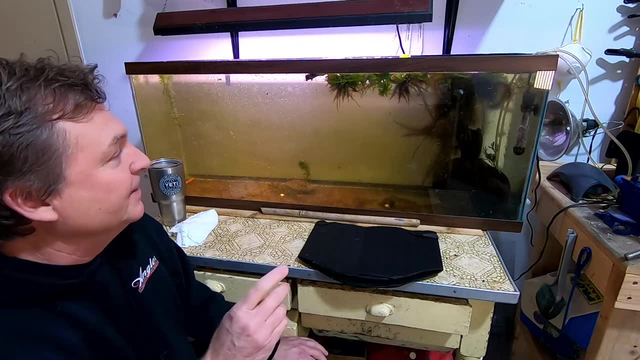 water and light and all that. i do have a light on it on a timer here, but i've messed around with and more light and they seem to still reproduce as long as they've got food. so if you don't give them food, they're gonna stop reproducing. and what would 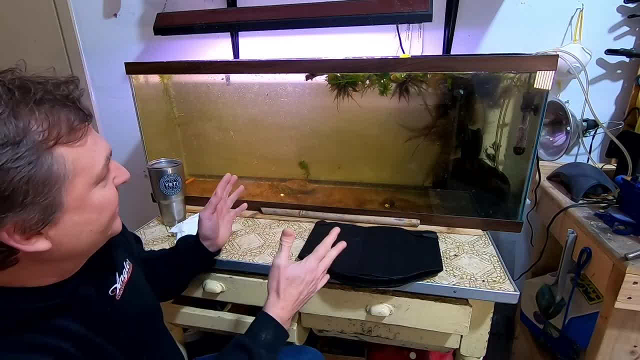 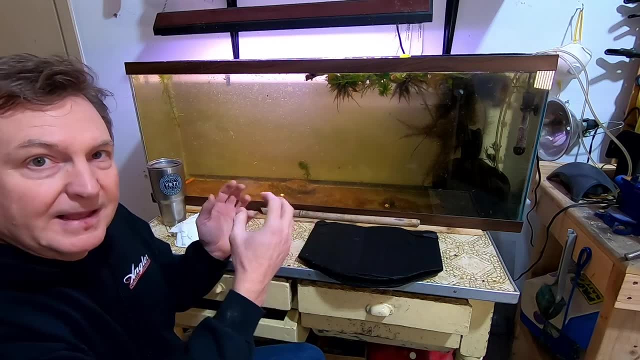 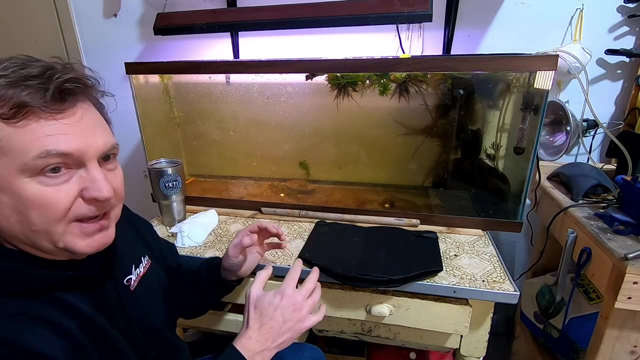 happen with this species. I've never haven't tried it, but they'll. some of the some of them will turn into males and they'll produce eggs through sexual reproduction. and there are different kind of egg. they're harder and they'll sink down to the bottom and they can survive through a cold winter or time. 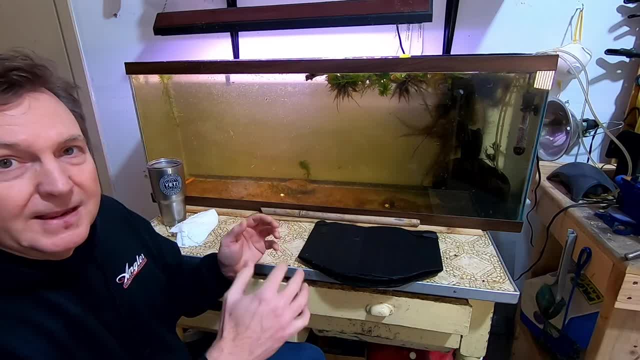 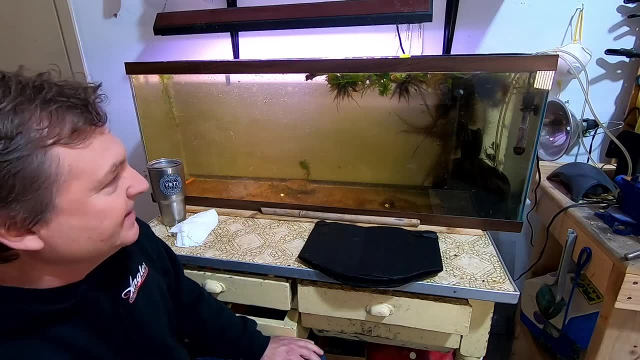 with no food, or if the pond dries up or whatever, and then, when the conditions are right, again they've got good water and good food- they'll hatch, and you've got Daphne. so they're pretty amazing when it comes to its survival. so what do? 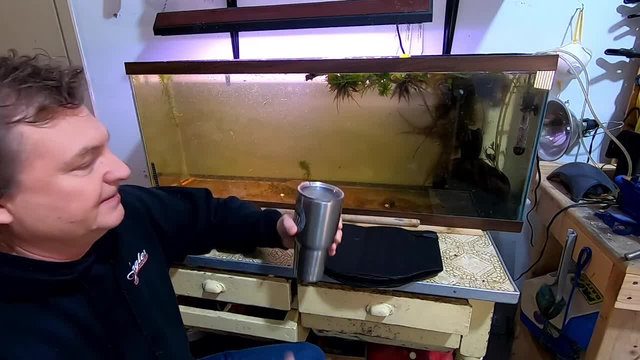 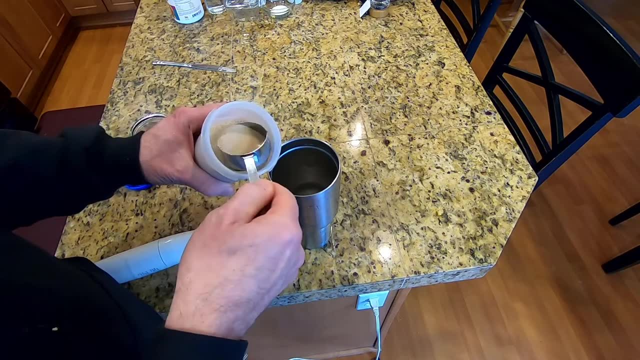 you feed them. well, what I've gotten- this little Yeti cup here- is ground up, let's say ground up. I've got a food processor, or a single like I'm. I think a magic wand is what they call it. I've got a food processor or a single like I think a magic wand is what they call it. 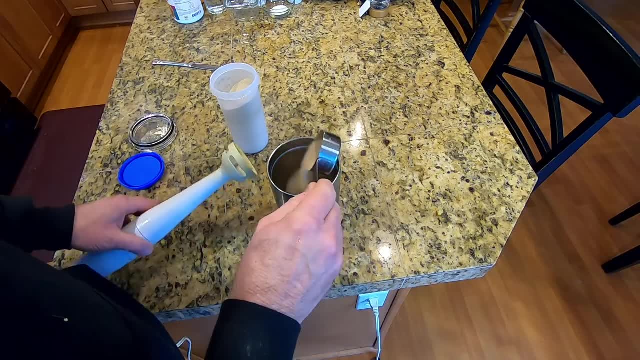 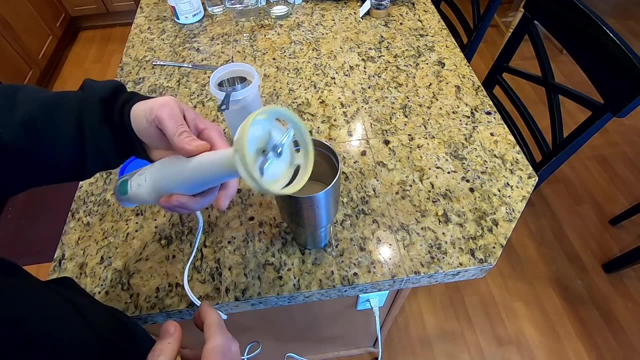 used to call them. it's something my wife had in the kitchen and it works great. but you take about a quarter cup of yeast, just regular yeast like you'd cook with, mix it in some water and just fill it up. look a little less than halfway when you're doing this, or else it'll splash around, make a mess, but kind of. 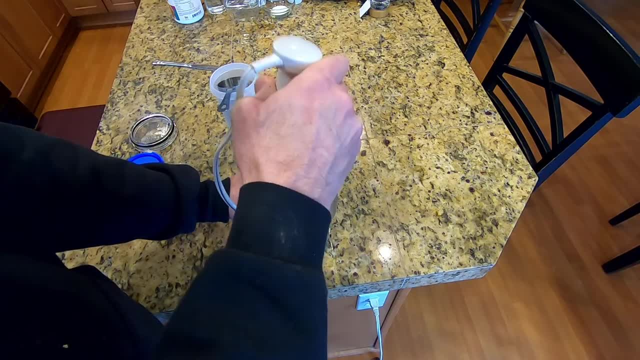 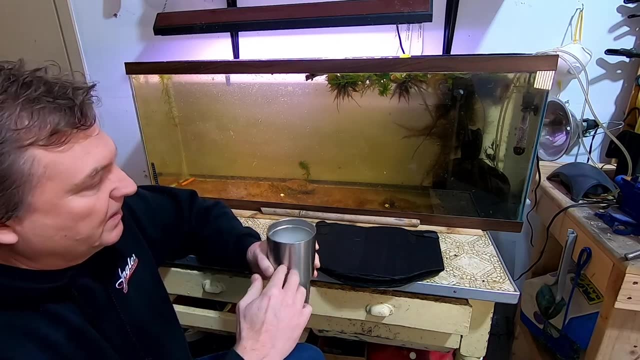 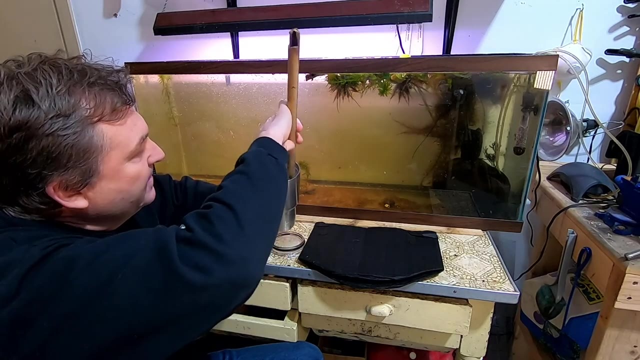 grind that into a nice fine slurry for them, and they're filter feeders. so then, after I've ground it up, fill up the cup a little bit more and keep it in the refrigerator. but I'm ready to feed. I'll just mix that up. good, because it will. 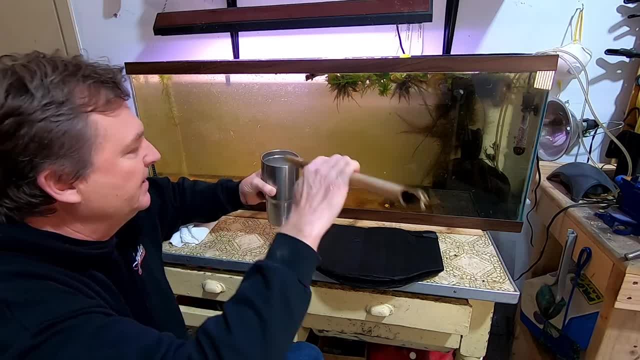 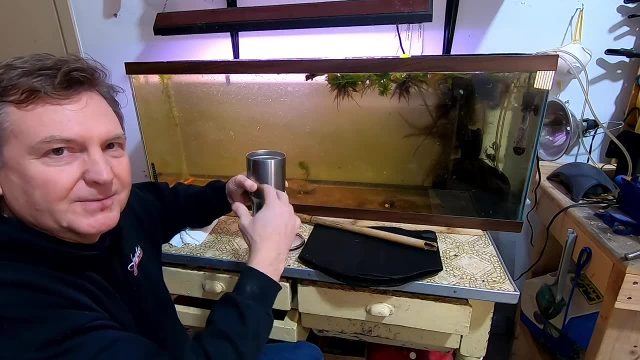 settle down at the bottom, and the reason I want to grind it up it's if you just put just yeast out of the package in there, it'll come, you know, float, and then it'll just sink to the bottom. it doesn't really mix with the water too. 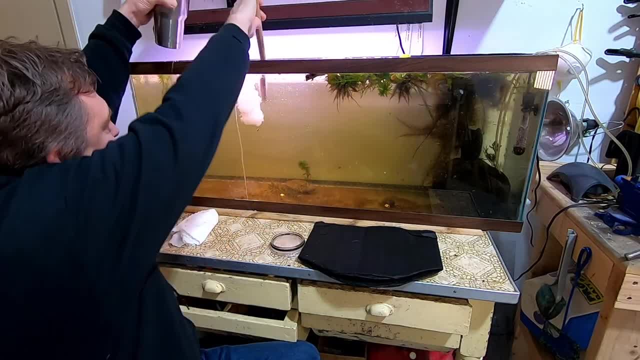 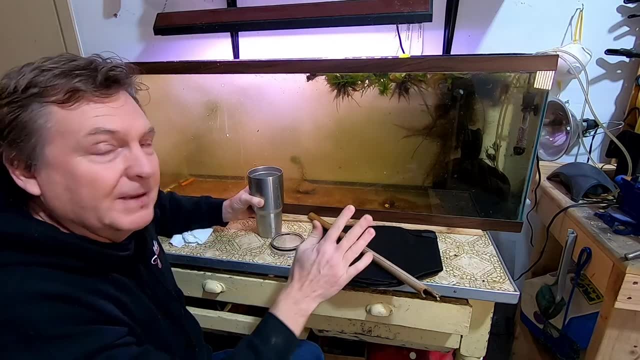 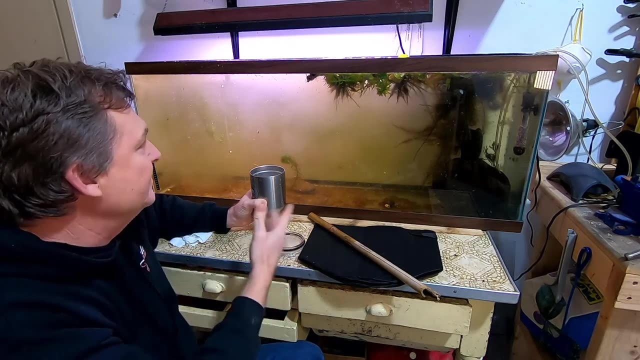 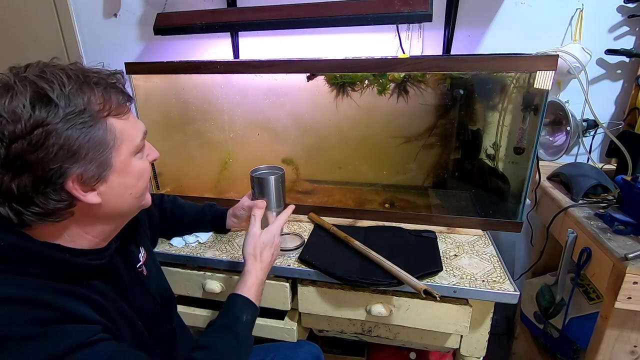 well, but then I'll just pour some kind of mist, just pour a little in there and mix it around, and you see, all that makes the water cloudy and that's what they eat. they're just gonna filter that yeast in and within. oh, by the way, the morning, you know six, eight hours to twelve hours probably. 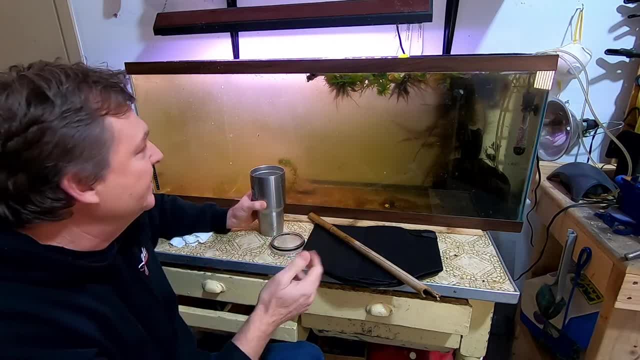 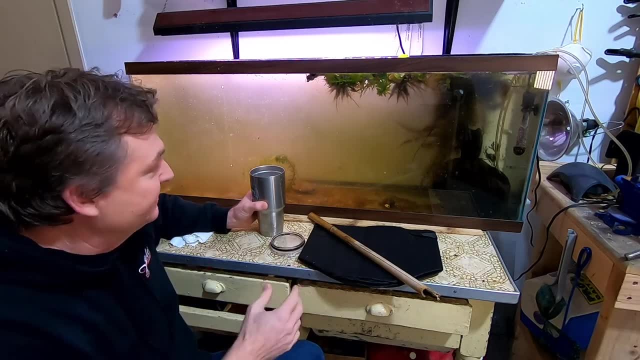 this water will be perfectly clear and you can feed them again. now the worst thing you can do is to overfeed them. that happened once I went on a trip and my wife fed him for me, and she poured way too much in there and I came back. 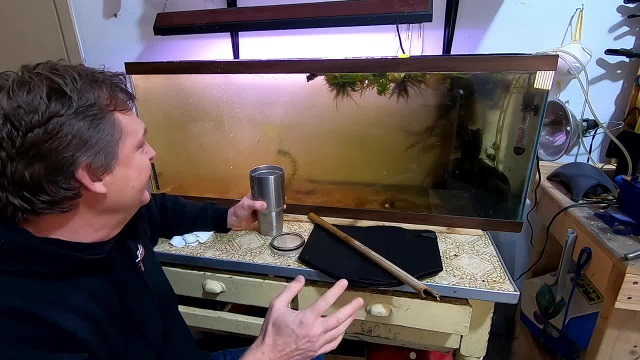 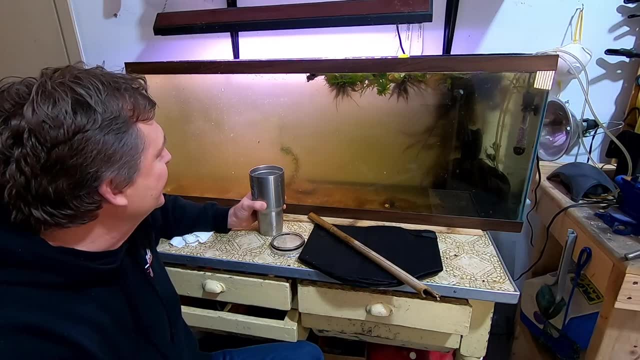 and I almost lost them all. I only had a few left in. there was like, oh no, I did a big water change and got them going again and it only took like a week and they were back to big numbers. so that was really cool. but yeah, you got to feed them, but don't overfeed them. so the food. 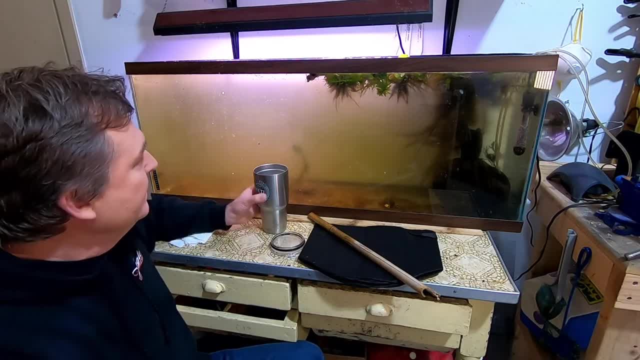 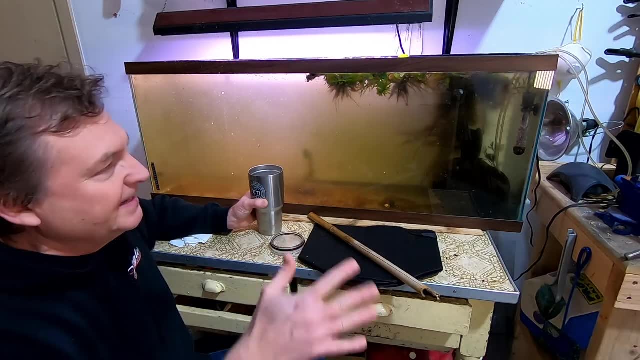 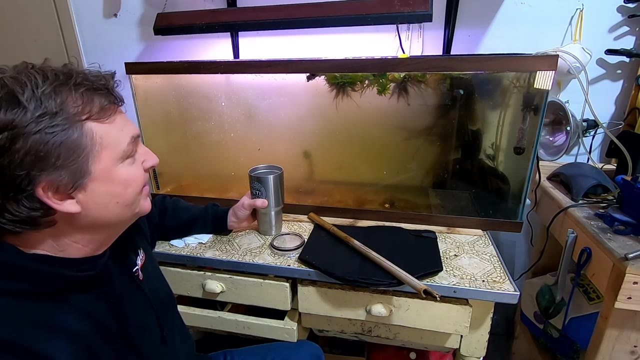 will spoil in there and, and you know, ruin the cycle. so, uh, yeah, I've. there's other things you can feed them. uh, besides this, I know a lot of scientists that work with these. they'll feed them alfalfa and spirulina and, uh, ground-up trout chow, that's a big one. so I think there's lots of things you can. 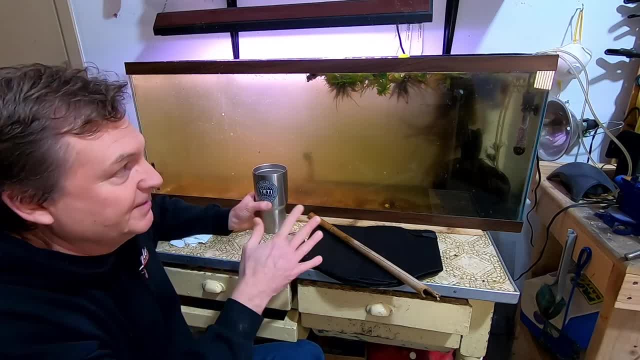 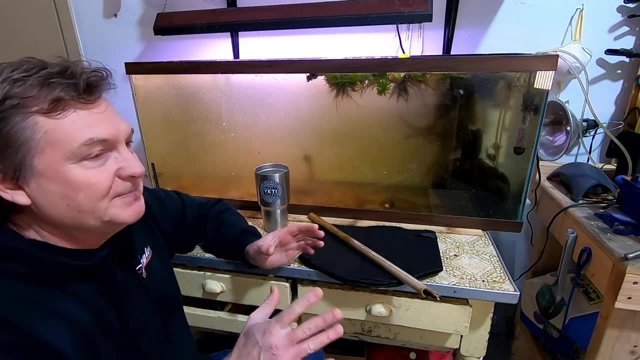 feed them. but besides the yeast, which seems to do well, I will give them green water out of the pond. and what I mean by green water is that so if you, if you look at the pond out there, if you look straight down in the water, it looks. 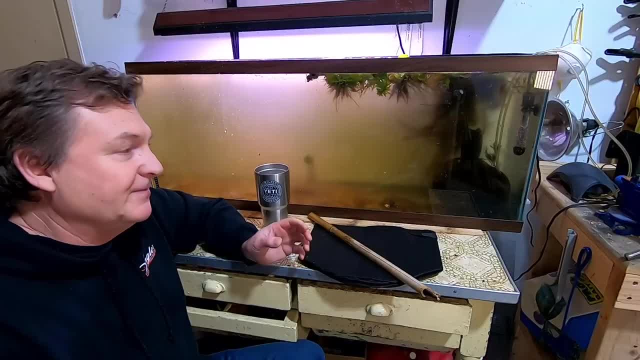 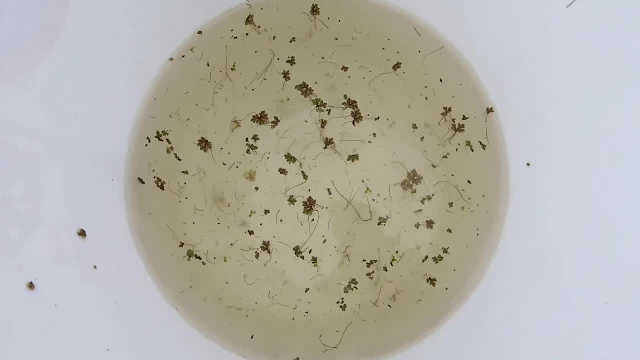 perfectly clear. the water is just amazingly clear. but if you take that same water and put it in a white bucket, you can see how it's kind of green. now it's the middle of winter right now, but in the summer that water will even be greener because that the greenness in there is algae. basically it's, it's. 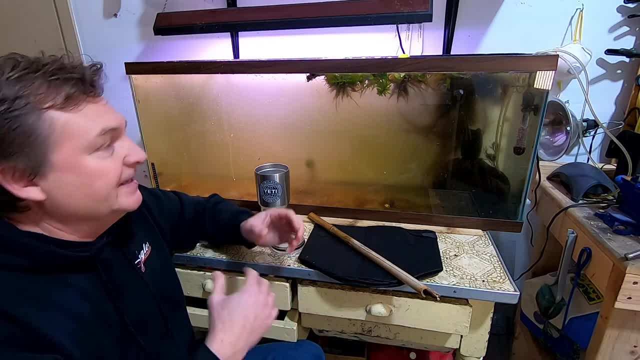 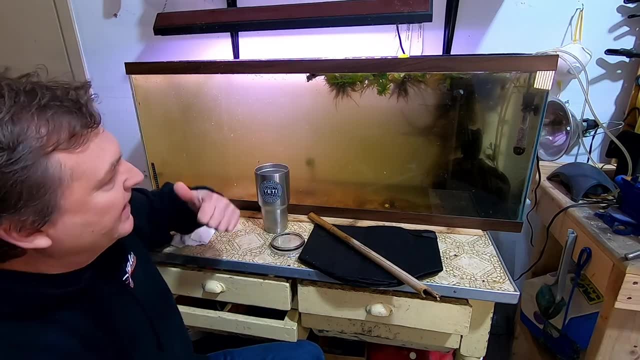 phytoplankton and algae. that's what makes it green and that's a real natural food that these guys really like. so, about once a week I'll take five gallons to siphon five gallons out of here. take five gallon bucket, bring some water in. 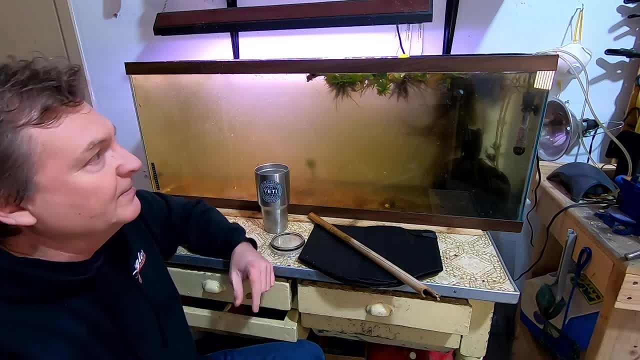 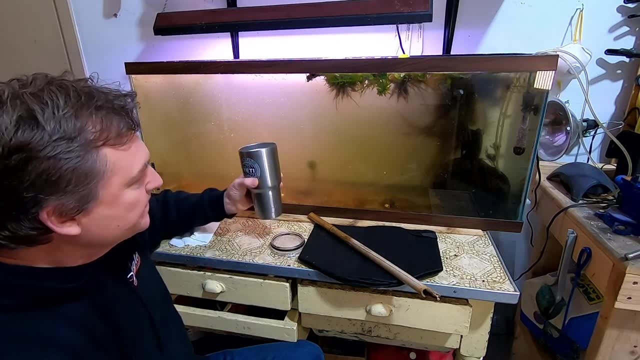 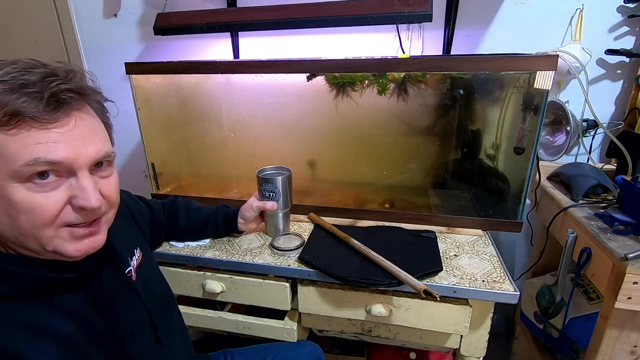 from the pond and that's a real treat for them. that's a little water change on the tank and everybody's happy and good to go, and otherwise I'll feed them the yeast about you. well, at least once a day, but twice a day. with its best, I think a little bit twice a day is the. 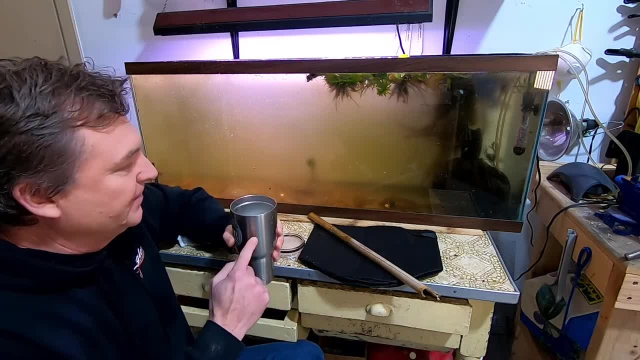 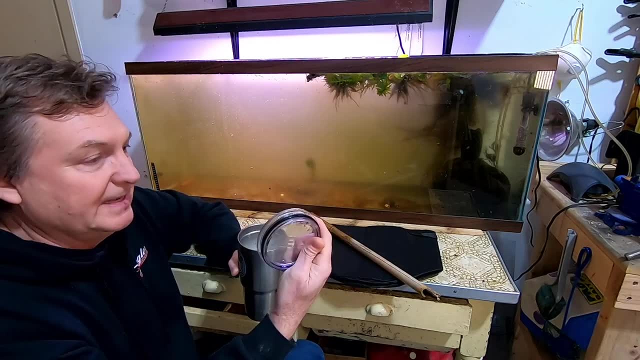 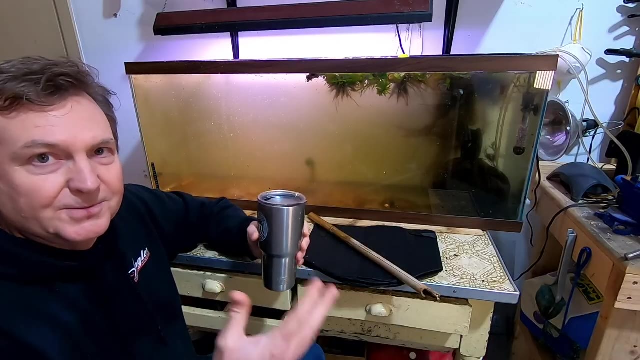 way to go. now the cup here. I'm using this cup for a reason: it's metal and I can do the grinding in it and it also. I love this lid because it's got a hole in it. you know, with yeast it's still alive. if you, it's going to do what yeast does.